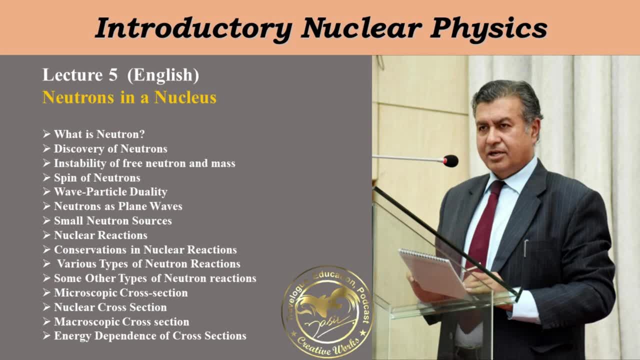 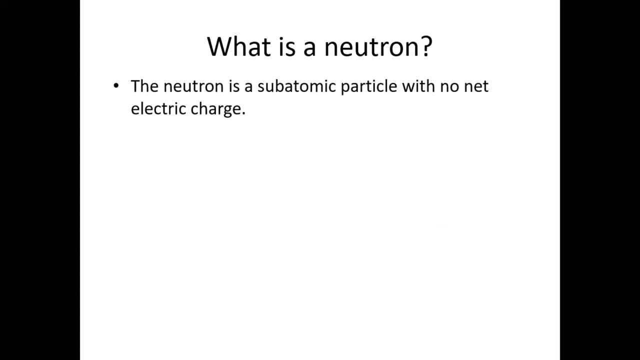 We start today's talk. I am Dr Nasir Majeed Mirza and this is introductory nuclear physics, and today's topic is the neutrons in the nucleus. What is a neutron? Neutron is a subatomic particle with no net electric charge. Neutrons are bound within the nucleus through strong nuclear force. 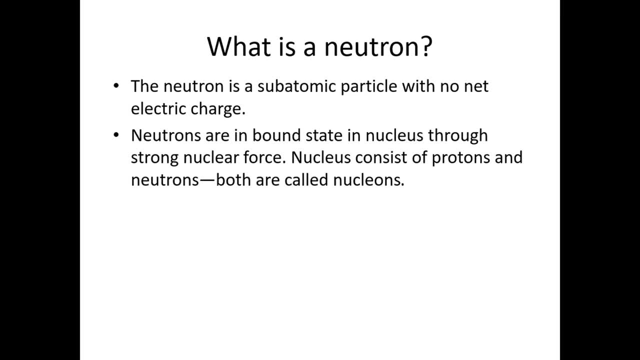 In coming lectures we will discuss in detail what is nuclear force, the strong nuclear force and the weak nuclear force. The nucleus consists of protons and neutrons, and both of them are termed as nucleons. The number of protons determine the element and the number of neutrons. 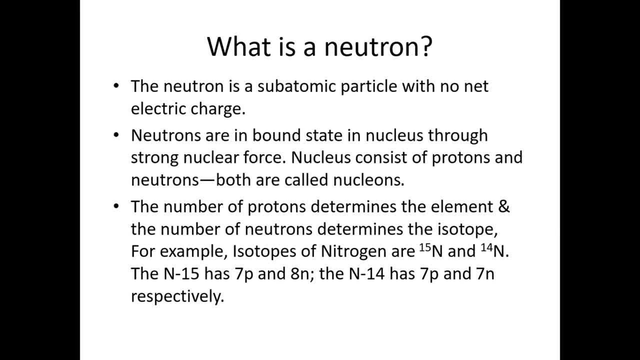 determine the isotopes. For example, isotopes of nitrogen are the nitrogen-15 and the nitrogen-14.. The nitrogen-15 has 7 protons and 8 neutrons. However, the nitrogen-14 has 7 protons and 7 neutrons. 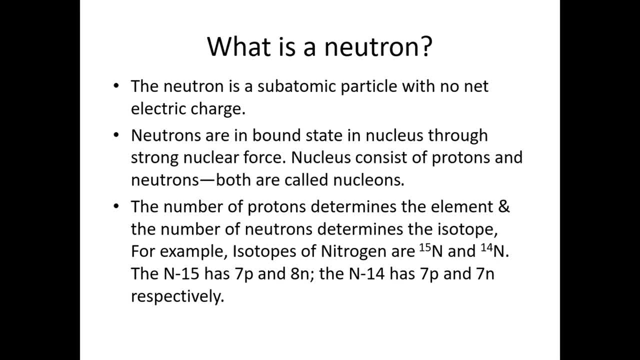 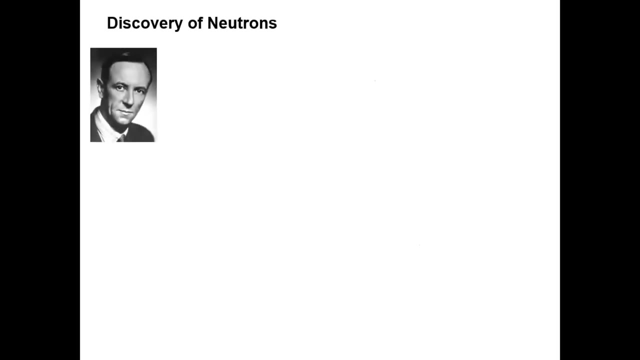 So you can see that the change of the number of neutrons is going to dictate the isotope nature, and the number of protons within the nucleus decide about the nature of the chemistry of the element. Let's briefly discuss the neutron's discovery. in 1920s, Rutherford postulated that there were 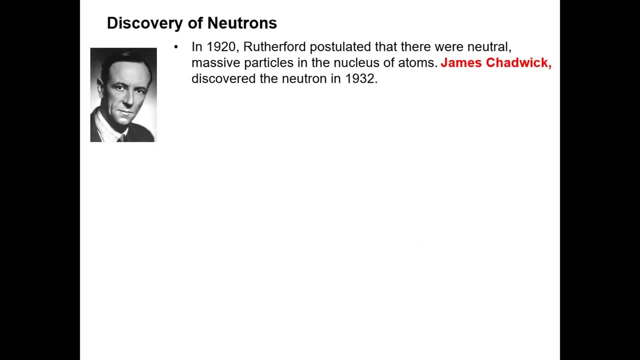 neutral massive particles within the nucleus because the mass of the atom is larger. as we see it, cannot be just the protons. James Chadwick discovered neutrons in 1932. He bombarded beryllium target with alpha particles and produced neutrons that recoiled into a block. 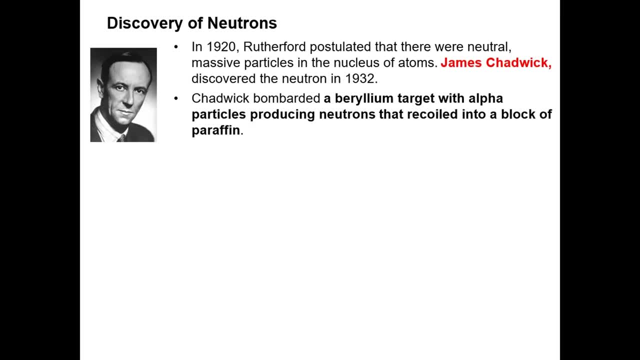 of paraffin wax. Paraffin wax contains carbon and hydrogen in a complex molecular structure, But for carbon there are four hydrogen atoms and therefore so many protons are available, and the alpha particles were producing the neutrons that were recoiling in the block of the paraffin. 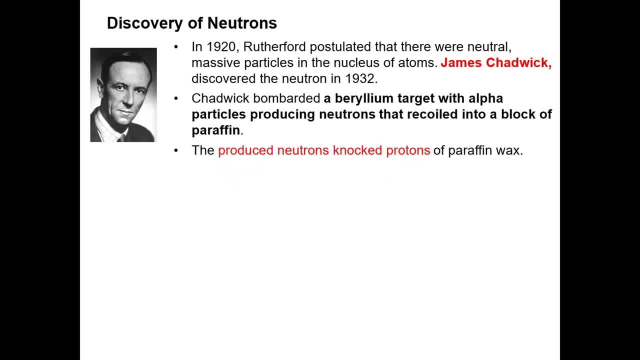 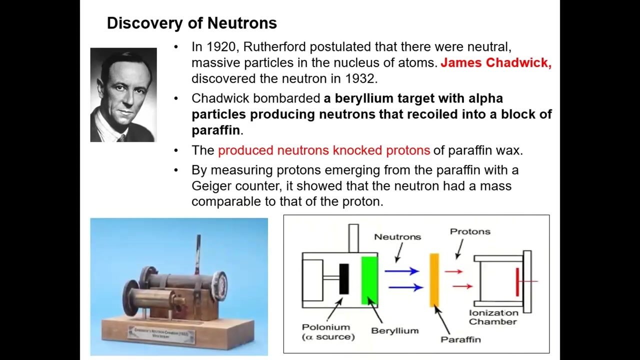 The produced neutrons were knocking the protons within the paraffin wax. So, measuring the proton emerging from the paraffin with the help of a Geiger counter, he showed that the neutrons have mass comparable to that of protons. If we look at the simple schematics of 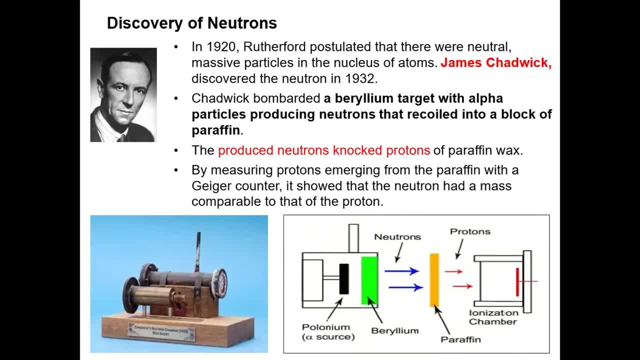 the of the experimental setup. then we see that the first is a polonium source, which is an alpha source. it emits alpha particles and in front of that the beryllium is placed. So the reaction, the nuclear reaction, takes place. As a result, neutrons are emitted and these neutrons travel towards the paraffin. 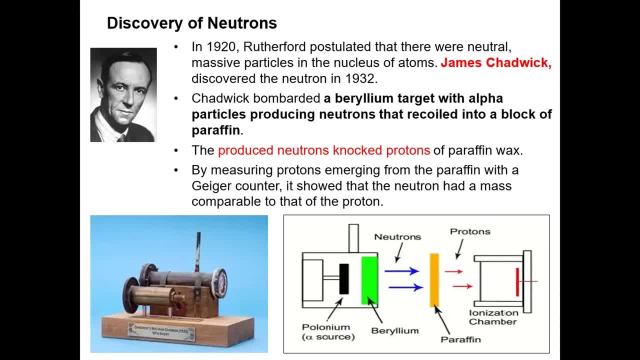 So in paraffin neutrons collide and scatter and this scattering produces the protons. It is kind of sort of a weird ball game in which the neutron hits the protons. Proton-rich environment is paraffin and these protons are really going to the ionization chamber, or 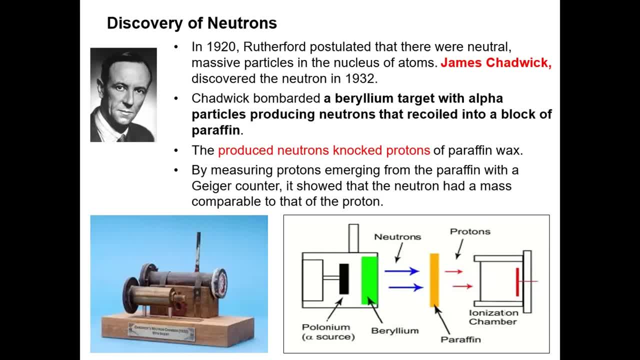 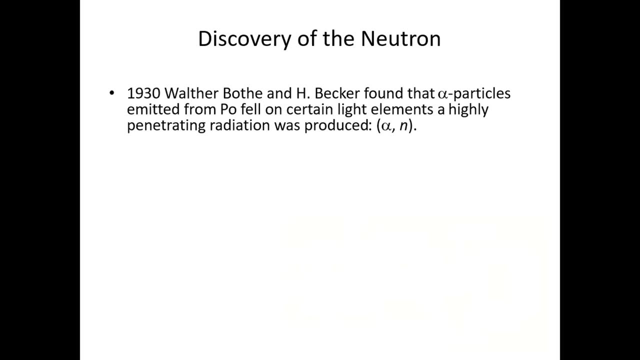 the Euler-terminal. It's going to try to force the minutes. just get rid of these protons, the 酵m´a, and then they are. other was her alpha particles emitted from plonium. They, when fall on certain light elements such as 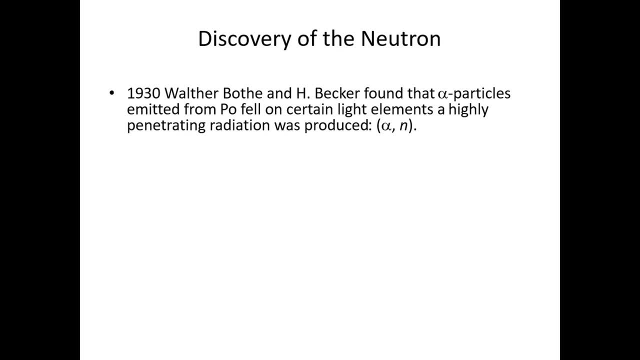 beryllium, then they produce very penetrating radiations and eventually we came to know that it was alpha n reaction. Alpha particle is the incident particle and the emitted particle is neutron. In 1932, Irene Julio Curie and Frederick Julio showed that this unknown radiation, which is 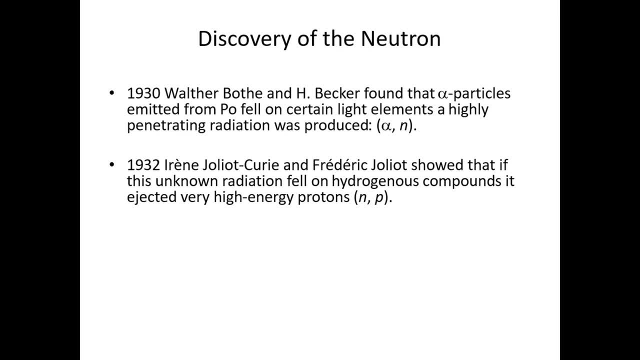 falling on the hydrogenous compound. it is ejecting very high energy protons. So they concluded that something is going on the neutron or something is hitting and the protons are getting out. They calculated originally the energy and it was not really correct energy distribution. 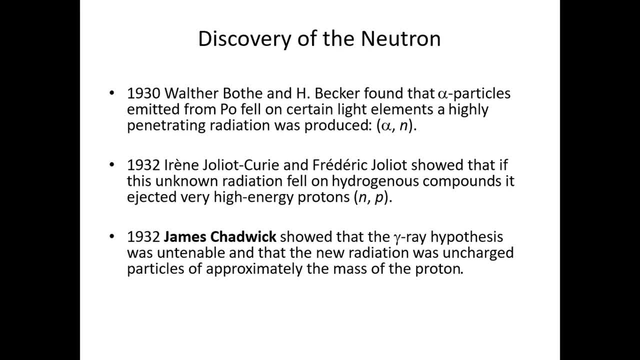 that was possible and therefore their idea was rejected. They said that it is a very strong gamma rays and that idea was also rejected. In 1932, James Chadwick showed that the gamma ray hypothesis of the paper written by Curie and Julio was really not. 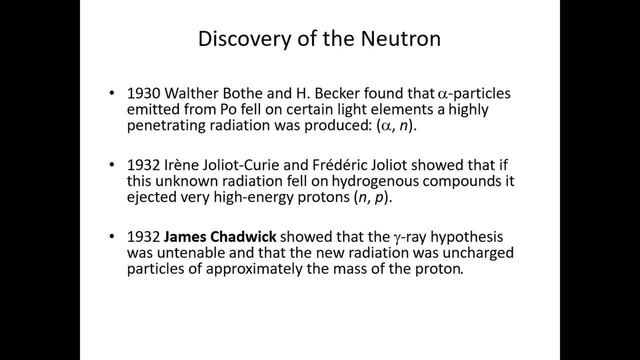 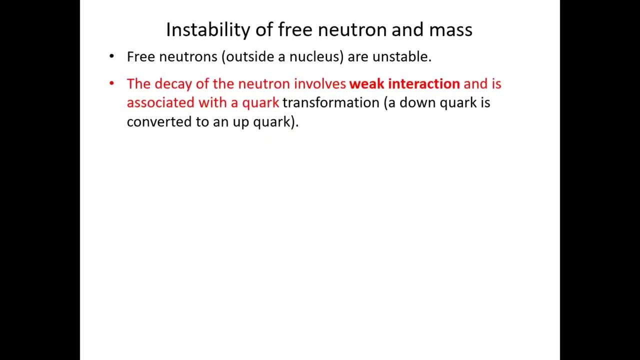 the correct version and the new radiation that was coming out was uncharged particles approximately that of the mass of proton and that led to the discovery of the neutron. If we go through the certain properties of the neutrons and we see that the free neutron is unstable and outside nucleus, it 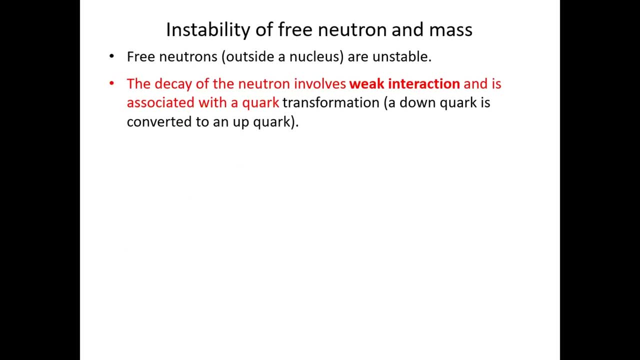 will decay. The decay of the neutron involves basically a weak interaction and it is associated with a quark transformation. A down quark is converted into up quark and that's what we know, know very well after the quark theory came and the weak interaction was thoroughly explained. 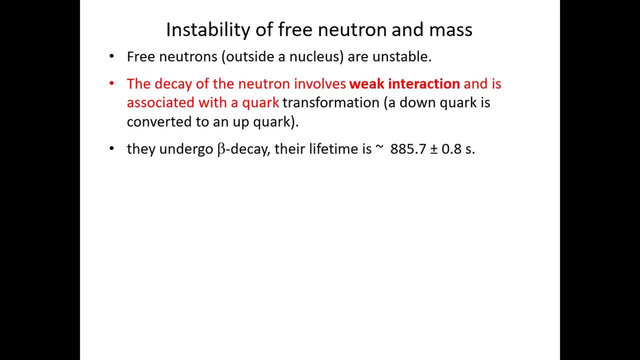 The beta decay, in this regard, can be achieved by a kind of�. the beta decay, in this regard, can be achieved by a kind of ginkgo nut creates approximately a lifetime of 885.7 seconds, with plus minus of 0.8 seconds. 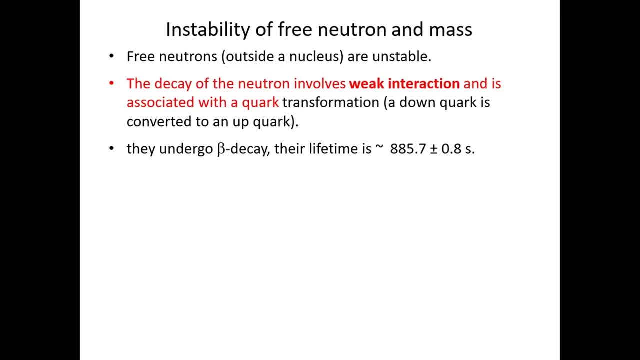 So it's roughly 885 seconds that a free neutron can live without nucleus. They cannot be stored long without the nucleus and outside nucleus they are going like this: A neutron is produced, then a neutron converts into a proton and electron and the anti particles or the idea of the neutrino. 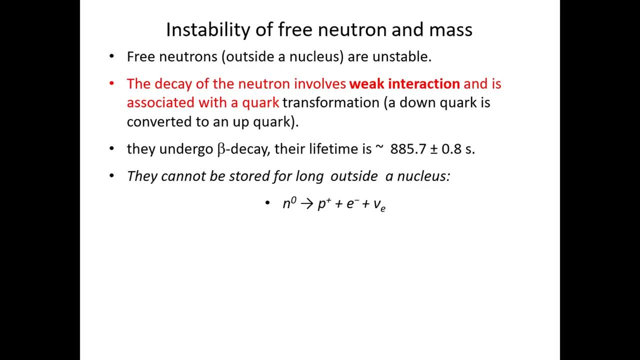 carrying energy later came, because it was very difficult to explain the beta decays energies, and the energy to spectrum was a continuous spectrum, It was not a discrete spectrum And therefore it led to the discovery of this neutrino, associated with this electron and the entire neutrino. 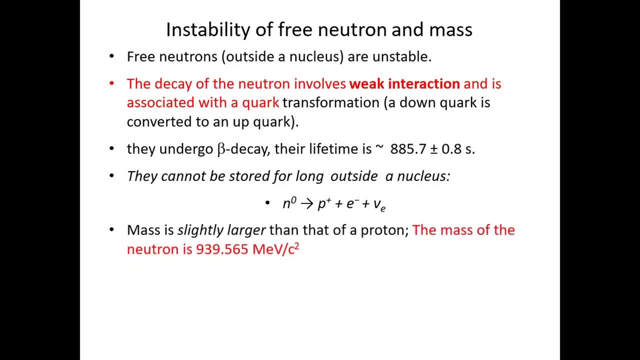 The mass of the neutron is slightly larger as compared to the proton in the mass in terms of energy is 9.565 million electron volts, according to electrona grid network method of material analysis, where the energy will be low and have desired, does not accept special neutrons. 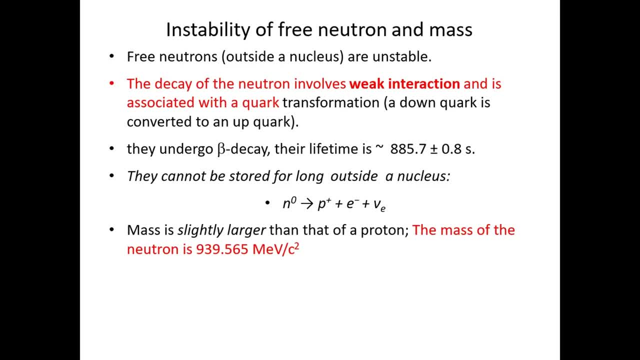 However, its iek performance is very good and energy is very good. Maximum level of infrastructure and portability. You can explain for the neutron. So here you'll have a small lots of нужengel match 0.5. Of electron volts. just wow, two games of salt: 5 and 4ol. 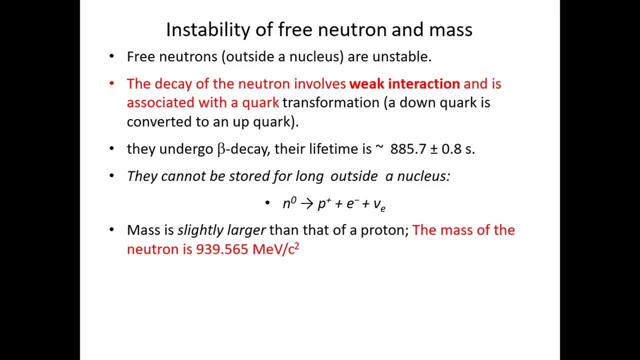 Then also a very dominant and a factional tet moth lower than ordinary electron problems such as potassium volts per c square. This is the current unit for the mass. Newtons have spin half, So they are spin half particles and according to modern statistics, 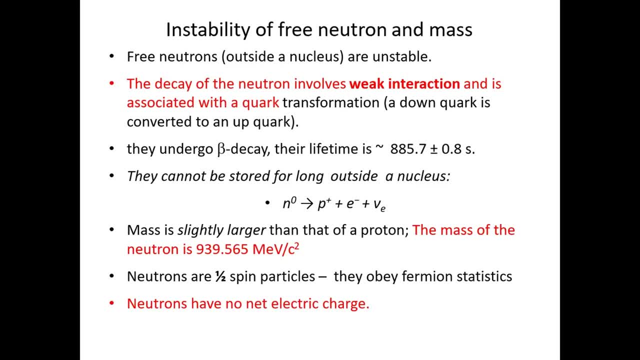 they obey the Fermi Dirac statistics. So they are fermions and the fermions obey Fermi Dirac statistics. and the spin half particles have certain properties that are really to be obeyed by the Pauli Exclusion principle as well. Newtons have no electric charge. Therefore, 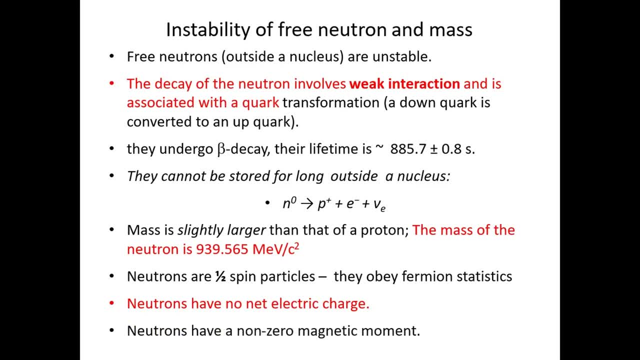 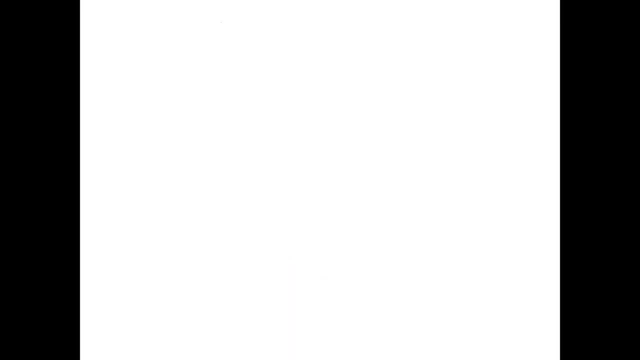 they remain neutral. However, the Newtons have magnetic moment. They have certain magnetic moment. in spite of the fact that they don't have net charge, electric charge, they have magnetic moment. The neutron spin is really very, very important. The spin quantum number S for the neutrons is half, So they are spin half particles. 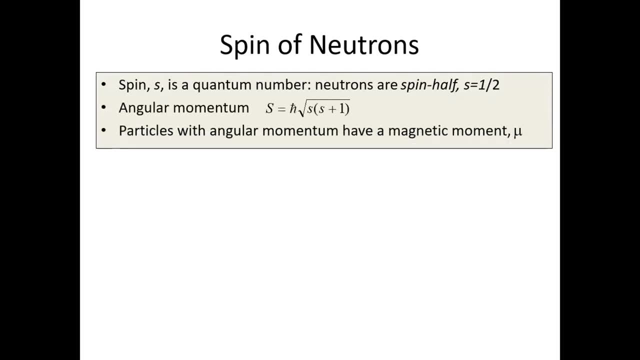 Their angular momentum is basically really can be can be estimated with the help of this equation, which states that it must be in the chunks of H-cut multiplied by under root of S into S plus half, S plus 1 and S is half, So angular momentum is really quantized and its value is half. Particles with the. 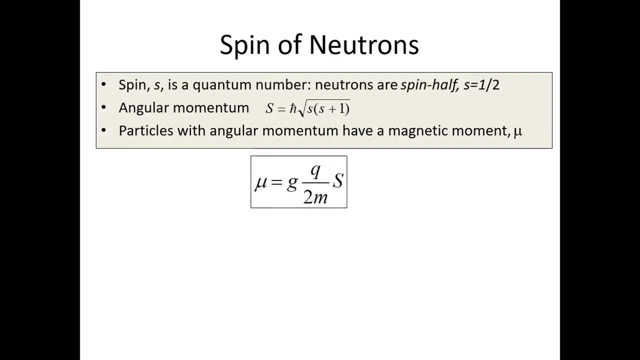 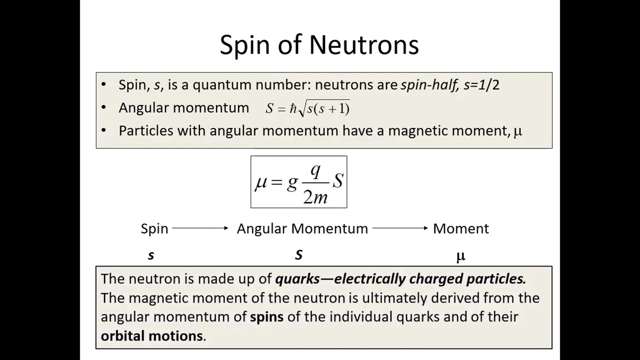 angular momentum have magnetic moments. So its magnetic moment is this: Although the net charge is not there, but the, this angular momentum's presence dictates. So basically, the spin is creating the angular momentum and the angular momentum results in the moment the magnetic moment. So neutron is really- now we know they are made up of quarks. 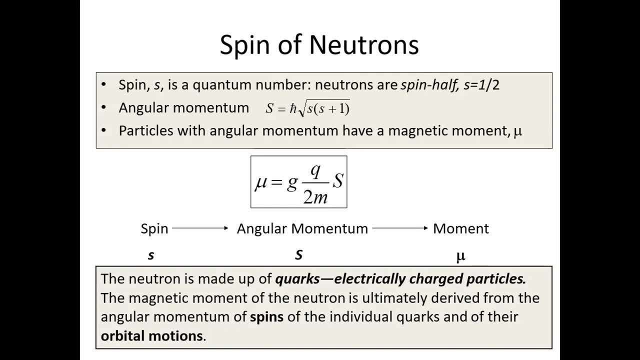 They are electrically charged particles. The magnetic moment of the neutron is ultimately coming as a result of the spins of the individual quarks, Because they have the orbital motions and they are really producing. So, although the net charge is zero, but the spinning quarks do produce the angular 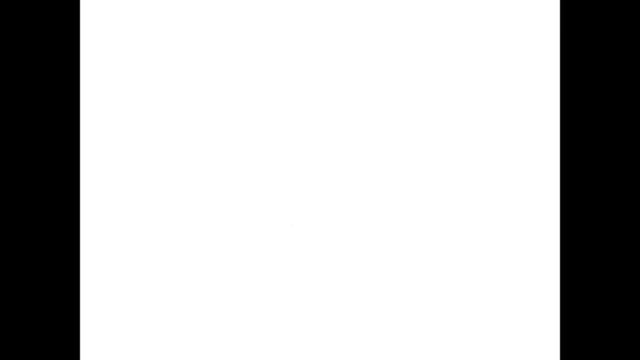 momentum and the moment. If I recall the wave-particle duality is intended to produce a tensile motion. Its De Broglie has already spoken on this- that every particle has an associated wave, So the neutrons, since all matter is wave-like nature. therefore the neutrons also have the associated wavelength. 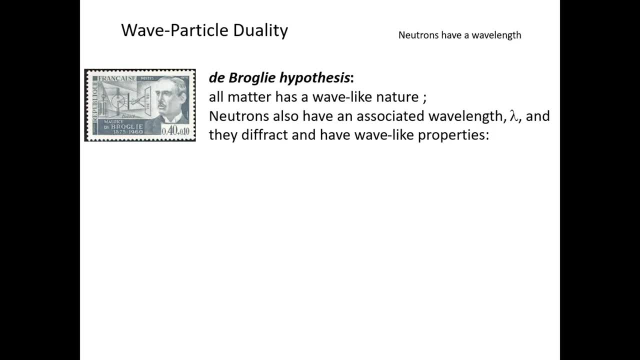 And they really show the direction and they have the wave-like properties And therefore they can show this: that energy is related to the frequency And the frequency is related to the wavelength And the wavelength is given by h divided by m into v. 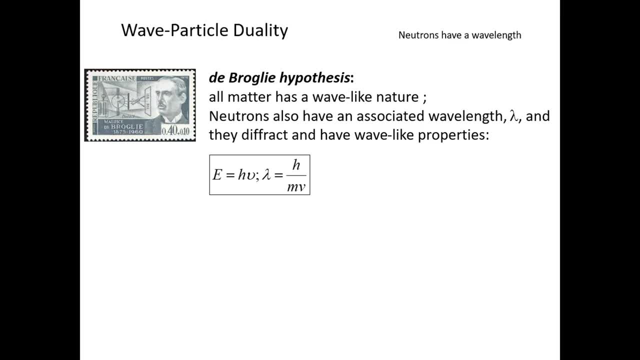 m into v is the momentum, the linear momentum. Therefore there is wavelength and there is frequency, And its energy relation can be estimated through this. The neutrons have wavenumbers, Since they have the wave, so the wave also have this wavenumber, which is defined as how many waves are really within the 2 pi. 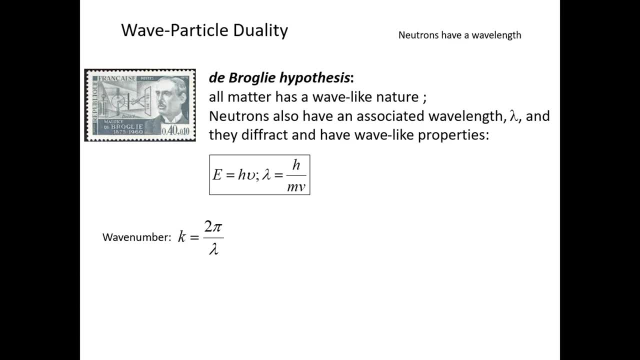 So 2 pi divided by lambda is the defining wavenumber. Strictly speaking, this wavenumber is the angular wavenumber because it is caused by the angular momentum of the neutron, And the energy in terms of the wavenumber is given as h cut square multiplied by k square divided by 2 m. 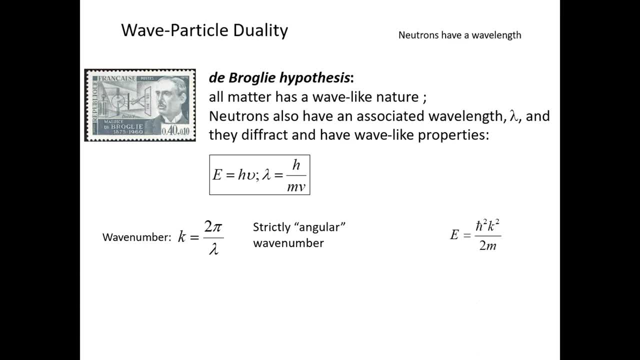 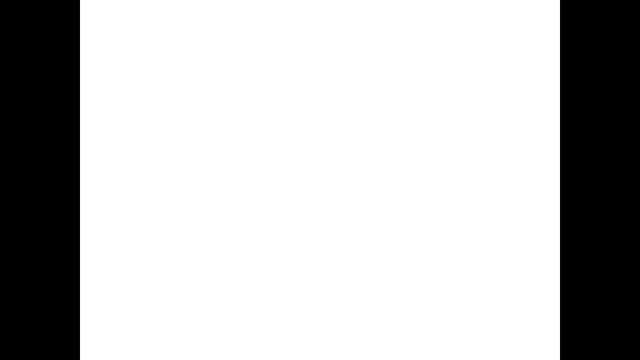 And that's how the neutrons are expressed in the quantum mechanics. Basically it is the wave Which has a wavelength and the wavenumber Neutrons really have plane waves. Constant frequency wave whose wavefront surfaces show a constant phase are infinitely parallel planes of a constant amplitude which is normal to the wave vector k. 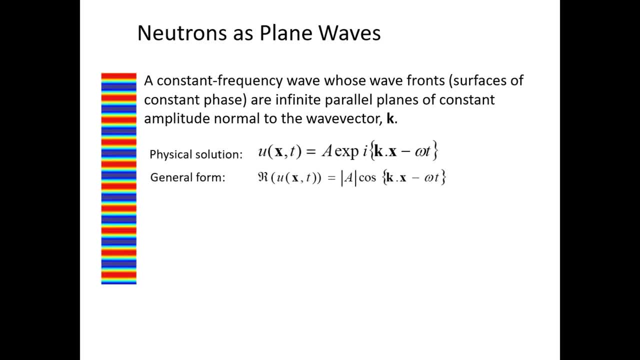 And if we want to write down in the quantum mechanics, we can show that the physical solution for the neutrons plane waves can be expressed in the form of this u, which is a function of the position vector x. It is not really the x coordinates, it is the x vector which has the x direction, the y and z. 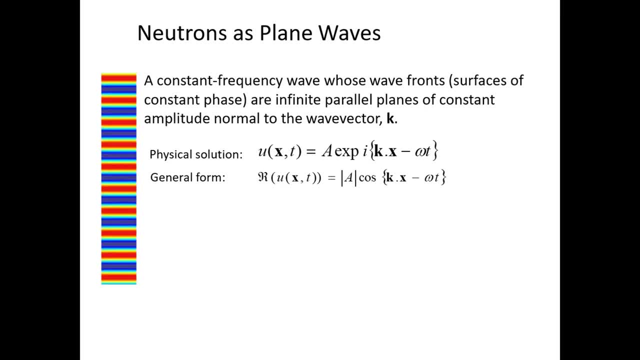 And the t And it is given as a Multiplied by e to the power iota times k, dot x, The k is a vector of the wave, vector which is perpendicular to the wavefront which is shown here, And the omega t. 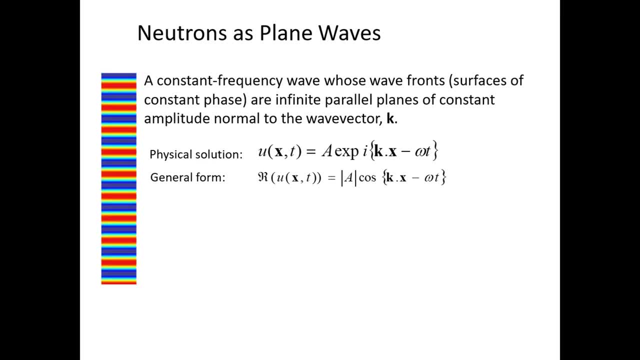 The omega is the angular frequency and the t is the time, And the general form for the such plane waves is given by a constant Multiplied by cos times: k, dot, x minus omega t, And it is the physically realizable wave. The k is the wave vector and the t is time. 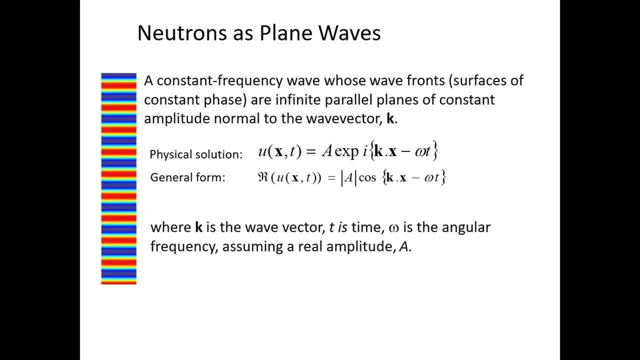 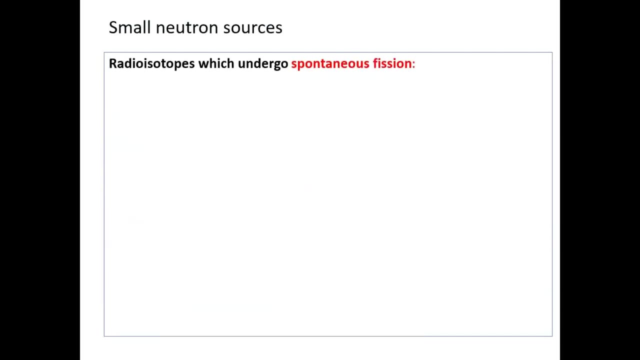 Omega is the angular frequency And we are assuming a real amplitude a, when it is the case And the neutrons really do have the plane waves because they have shown the diffraction. Let's talk about the Current situation, in which the neutrons can be produced with the help of the small neutron sources, and the first and the foremost source available is through the isotopes which can have the spontaneous fission. 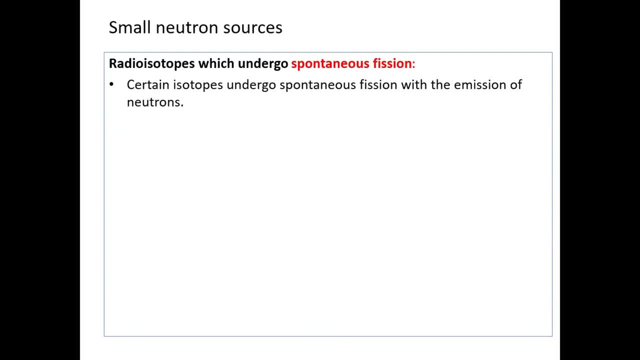 There are certain isotopes that undergo spontaneous fission with the emission of neutrons. For example, one fission source is the isotope californium 252.. It is a spontaneous fissionable source. It emits neutrons and typically californium 252 neutron source can emit 10 to the power 7 to 10 to the power 9 neutrons per second. 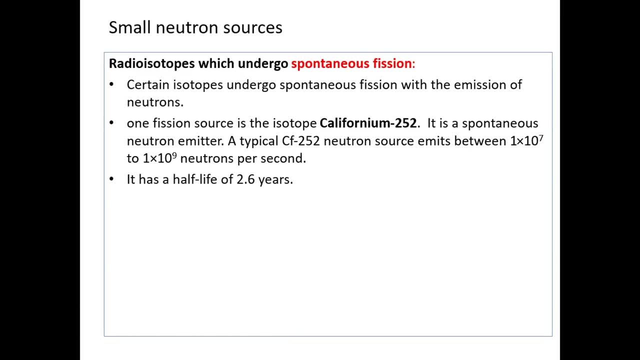 It has about 2.6 years of half life and it is only produced in nuclear reactors. Then there is a mission Beryllium type neutron sources that were originally used to produce neutrons in the discovery of the neutrons Emission. 241 emits alpha particles. 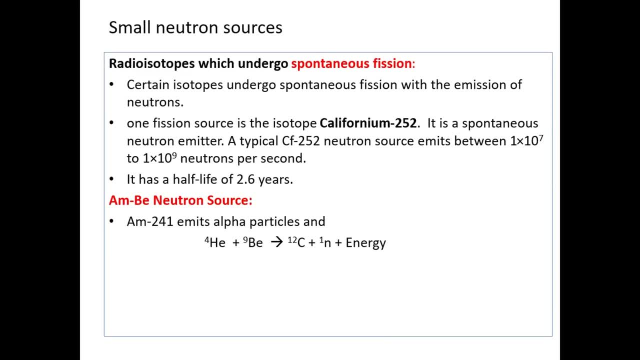 So this alpha, if it's going to hit the beryllium, then this nuclear reaction takes place. The combination of the helium and the beryllium nucleus produces C13.. C13 type thing Is such that it is, it is, it is unstable, and it then changes into carbon 12 and then a neutron and some energies released. the energy is the Q value of the nuclear reaction. 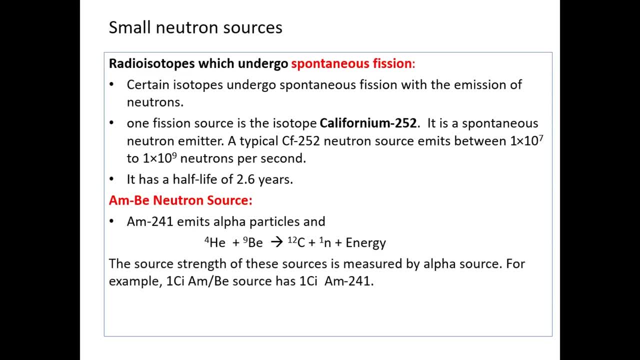 The source strength of these sources are generally measured in terms of the alpha sources. The larger the alpha source, the larger will be the emersion beryllium, Like neutron source. So, for example, if we have one Qd emersion beryllium source, then this one Qd source is basically due to one Qd emersion to 41.. 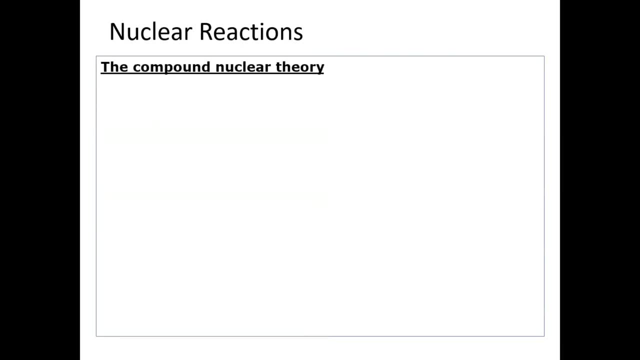 Let's briefly discuss the nuclear actions And how. because I have already shown you one nuclear reaction, I must brief you about the nuclear reactions. There is a theory which is termed as compound nuclear theory. We'll talk more about this in coming lectures, when I discuss the nuclear shapes and sizes and how the binding of the nucleus takes place. 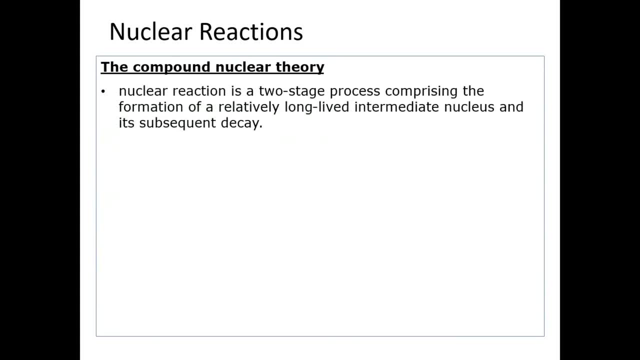 One idea is the compound nucleus, and a nuclear reaction is basically a two-stage process which produces first a relatively long-lived intermediate nucleus and then it decays into the parts that are really more stable. So a bombarding particle first loses all of its energy to the target nucleus and then it becomes an integral part of the unstable. 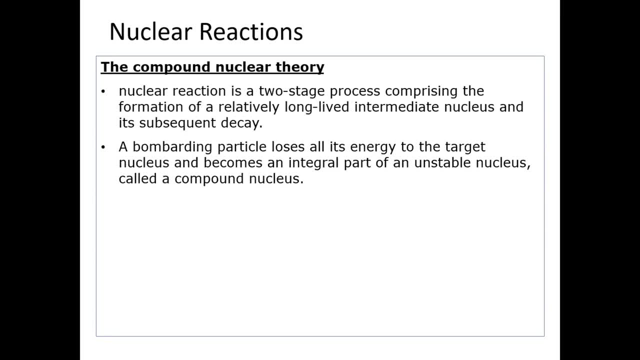 This nucleus is termed as the compound nucleus. The compound nucleus is really unstable. Then the compound nucleus disintegrates into two parts. One is the ejected small particle and then there is a product nucleus. So if we have X nucleus, the target nucleus, and A is the particle beam which is hitting this nucleus, then we produce a Z star. 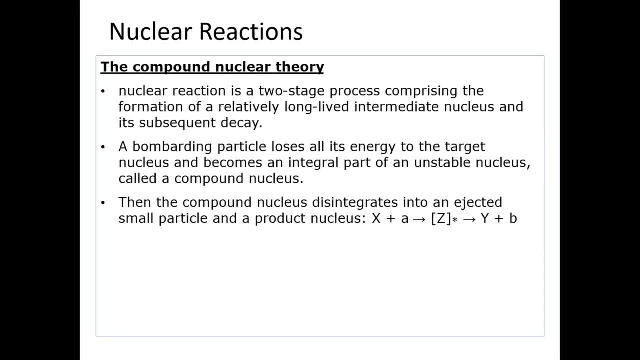 Something which is unstable, and then we get it converted into Y, a relatively stable nucleus, and then B, a small particle which is ejected out and going away. The compound nucleus is really the unstable, and this is this idea. The way it is generated is the compound nucleus theory and it was put forth by Niel Bohr. 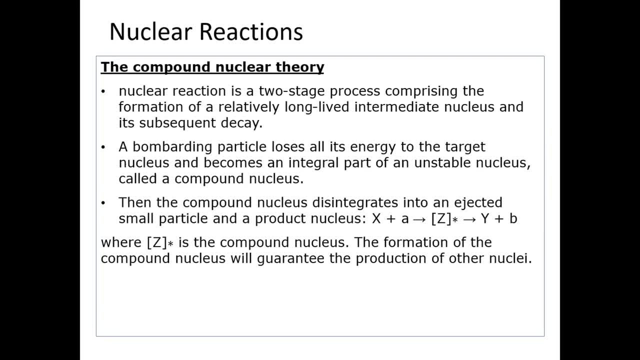 Bohr and still very useful for explanation of fission and fusion types of reactions. It, the formation of compound nucleus, then guarantees that the other type of the nucleus will be produced and something will be getting out In a nuclear reaction. there are several things that are conserved. 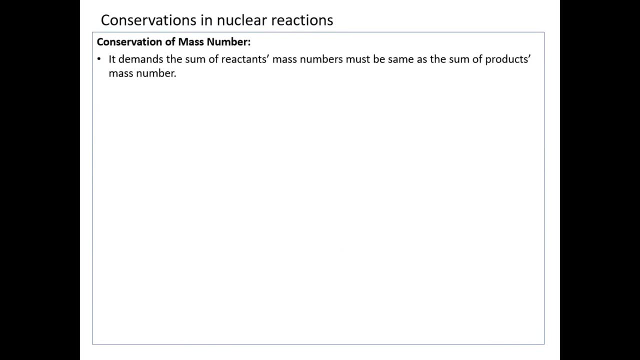 And if we go one by one, first conservation is that of the mass number. The mass number is the total number of the nucleons that are present in the nucleus. This number remains fixed. So the sum of the reactants mass number must remain the sum of the product mass number. 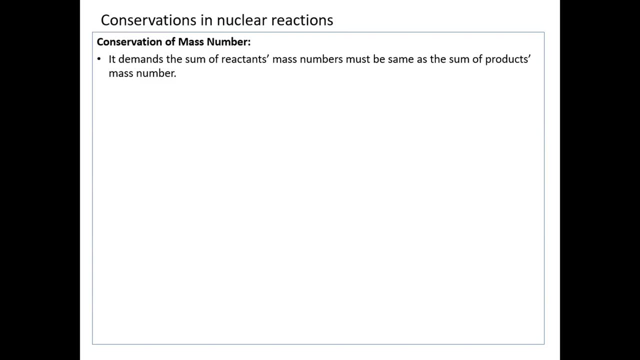 The original mass numbers and the final mass number remains the same. Then we have the conservation of atomic number. Atomic number stands for the number of protons or the number of charge, that is, the total charge Sum of the reactant, of the product. 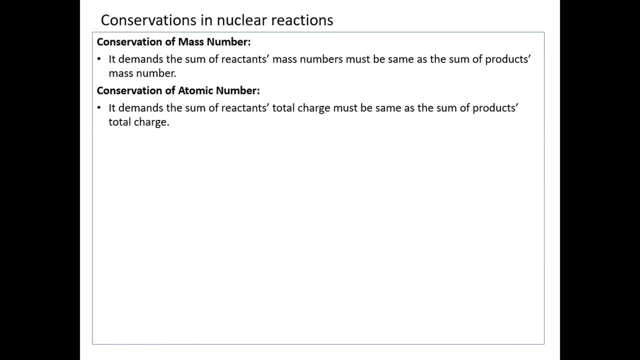 The total charge must remain the same. This charge is not going to go away somewhere. They are there. The conservation of energy is also one important feature. It demands that the total energy of the reactants must remain equal to the total energy of the products. 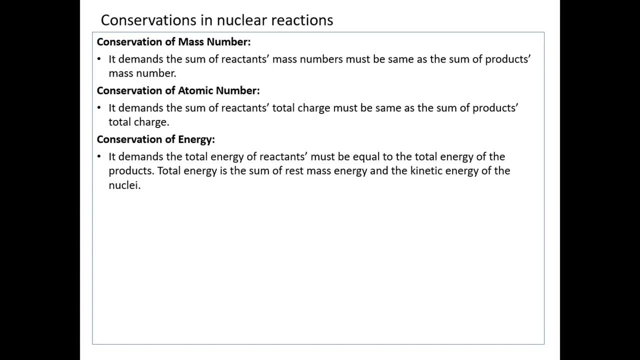 So the total energy is the sum of the rest mass energy and the kinetic energy of the nucleus in all these nuclear reactions. Whenever we are calculating the total energy, we must take into account the rest mass energy and then the kinetic energy. We will have several examples in coming lectures where we show this. 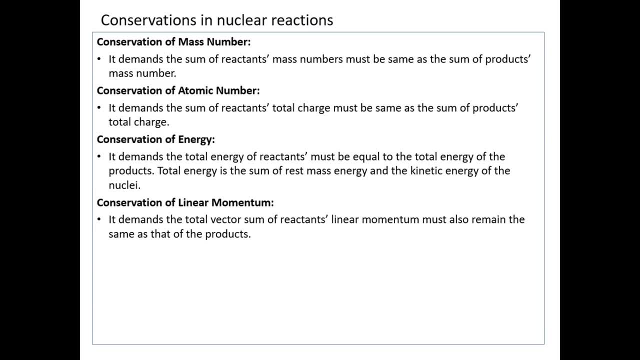 Linear momentum is generally consumed and it demands that the total vector sum of the reactant linear momentum must remain same Before and after the reaction. The angular momentum conservation is also Desired, that the total vector sum of the reactants angular momentum, which includes the spin, must also remain the same as the that of the product. 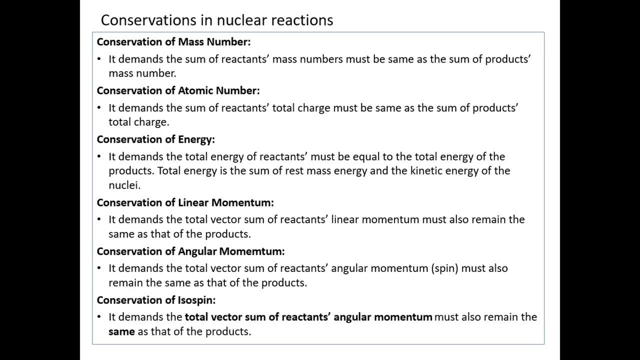 And the one another important idea is the isospin, which is demanding that the total vector sum of the reactants, angular momentum, the vector sum of the angular momentum, must also remain same, And this idea is called isospin conservation In nuclear action. 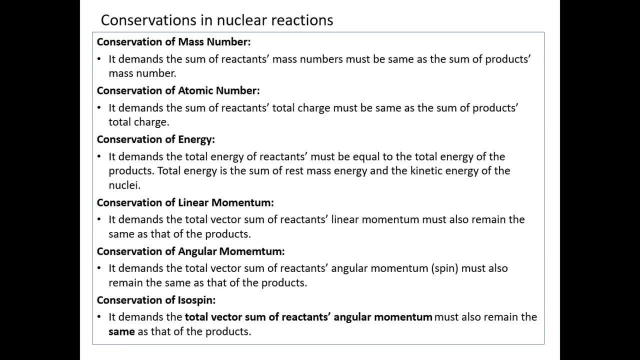 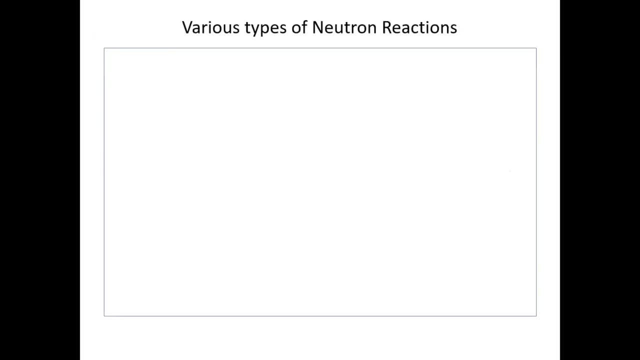 And can be processed if all these conservations are really obeyed, Let us look into certain details of the neutrons reacting With the nucleus. If we have produced a source of a neutron and we want to use use neutrons for certain nuclear reactions, we have seen that the neutrons generally do not 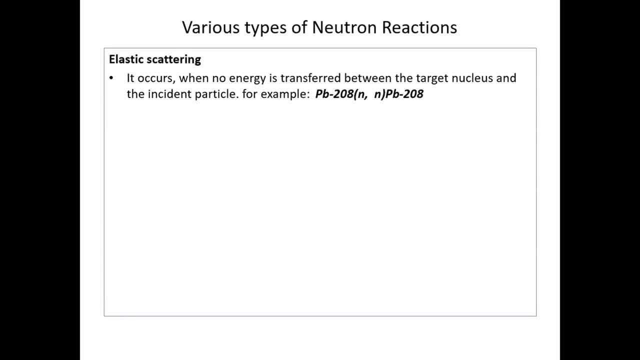 really show any reaction with the electrons outside the atom. They have tendency to have the reactions within nucleus. The first is the elastic scattering. It occurs when the no energy is transferring between the target nucleus and the incident particle, For example this lead PV208. 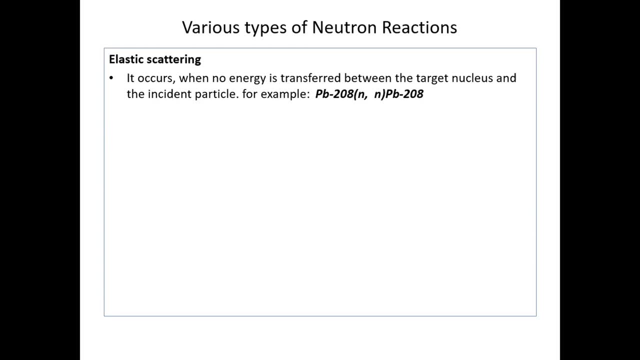 is hitting is hit by the neutrons and they are elastically scattered. Energy of the scattering is conserved. Then the neutron just scatters away and the lead nucleus remains the lead nucleus. Inelastic scattering is the case Which transfers the energy. when the energy is transferred to the product, For example, 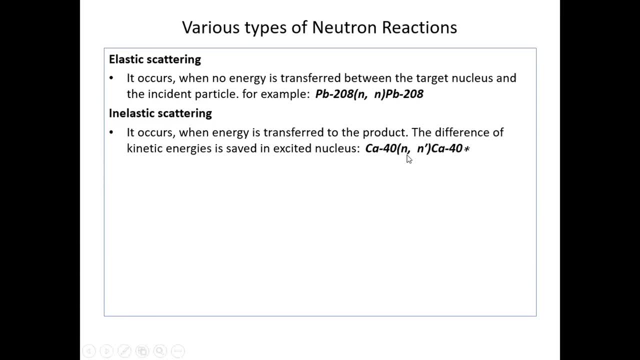 the CA40 is hit by the neutron. You can see this is the incident particle, The N is the incident particle and CA40 is the target on which it is hitting. When it is hitting, then it creates a compound thing and then their compound thing changes into CA40 star, which is the different. 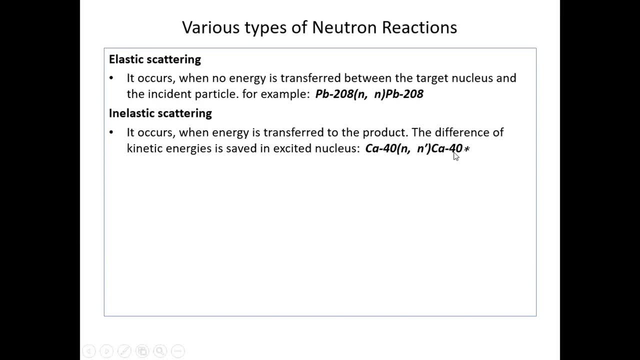 nuclear reaction. This is because it is in an excited state now And when it will de-excite it will emit certain form of energy And the N dash is also the neutron which is produced, which is coming out. And it is not the same neutron. It is with the different energy going in certain different 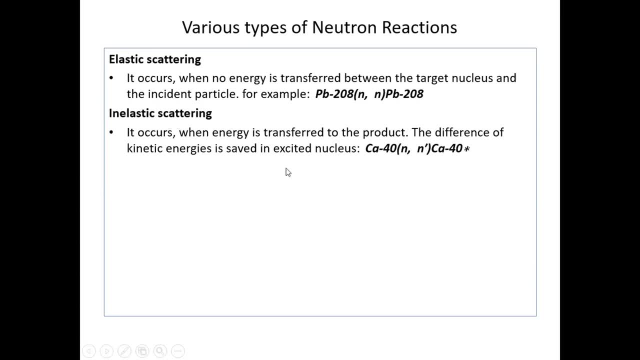 direction And therefore this reaction is the inelastic scattering. Then there is a capture reaction. Both charged and neutral particles can be captured. The nucleus can capture them, which means that once nucleus has captured the particle, it will only emit the gamma rays. Neutron capture reactions are very important And one important nuclear 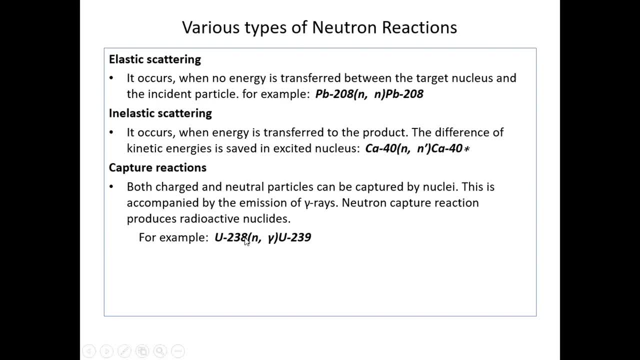 capture reaction is shown here. It is U238, which is hit by the neutrons And it is producing the U239 and the gamma ray. So the product is U239 and the gamma ray is emitted because when a compound nucleus was formed, it de-excites by emitting a gamma ray. So the neutron 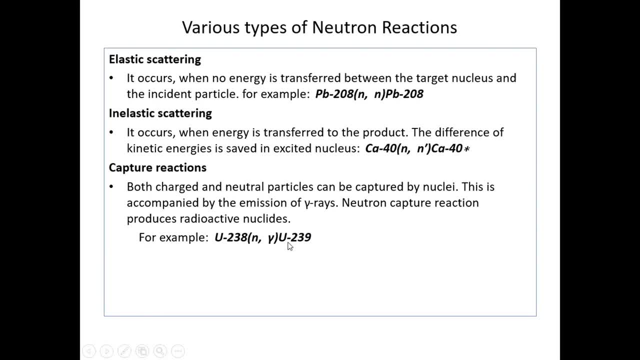 is captured and now the total number is changed. But uranium is uranium, 92 is the same, The Z number is the same, The charge is the same. Eventually this is unstable. It will decay into certain things and it becomes plutonium 239 eventually, And that we are not really showing here. 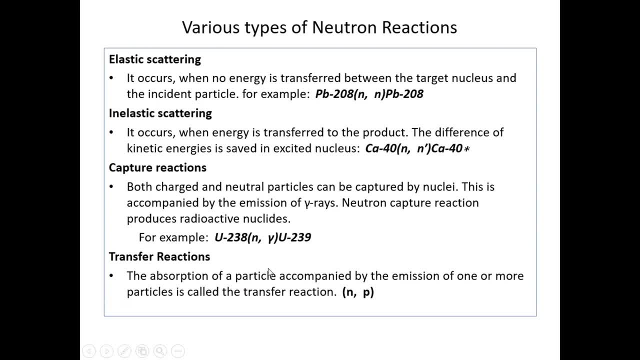 The transfer reaction is one important reaction in which the absorption of the particle takes place, But the compound nucleus emits one or more particles that are different. So concentration, these again myaldry of fast happening- risks occur. So the reaction here is a transfer reaction, A vertical reaction. 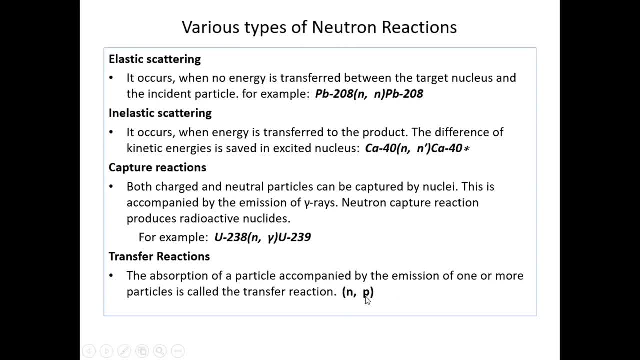 that is not Connecticut transfer, but the回 is Sp morpho reaction as I start to talk. So it is the transfer reaction and it is a transfer reaction. For example, Np reaction is a transfer reaction. N alpha reaction is a transfer reaction. 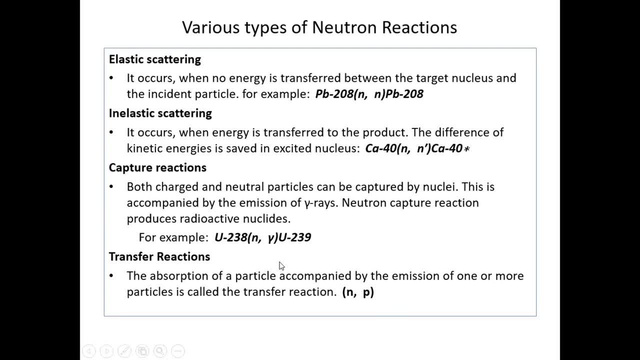 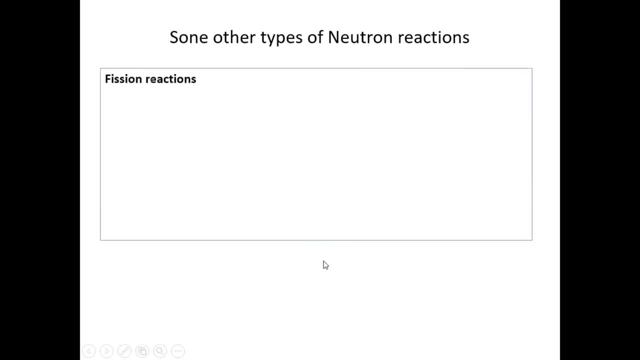 transfer reaction is accompanied by the emission of one or more particles. Some other types of nuclear reactions are also of interest in the nuclear physics, and one interesting reaction is the fission reaction. Nuclear fission is a reaction in which a neutron emitting the uranium-235, splits it into this lighter nuclei more than one particle. 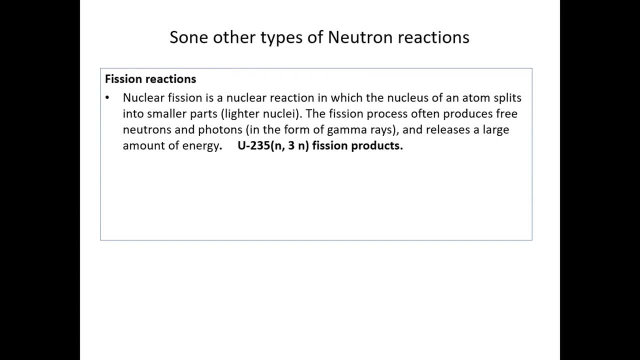 is, as a product is produced, two or more particles are produced, and we have seen that two or three neutrons are also produced. So those two or three particles that are eventually produced are called fission products. So the fission process processes in the nuclear. 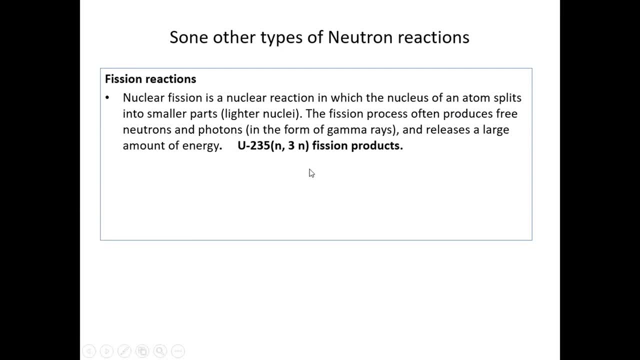 in which a free neutron or a photon will hit the uranium-235 and will release a large amount of energy and will produce two or three neutrons and the fission products. These two or three neutrons are really responsible for carrying the chain reaction, and that's why. 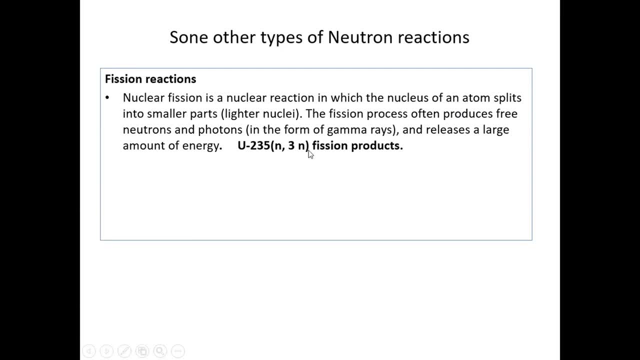 the fission reaction has become immensely important because it can. it can start flowing because one neutron is lost but the three neutrons are produced and there is those two or three neutrons can hit again and will keep on coming on, increasing the nuclear fission. 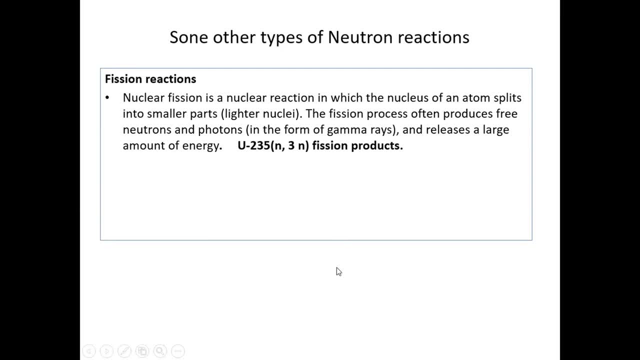 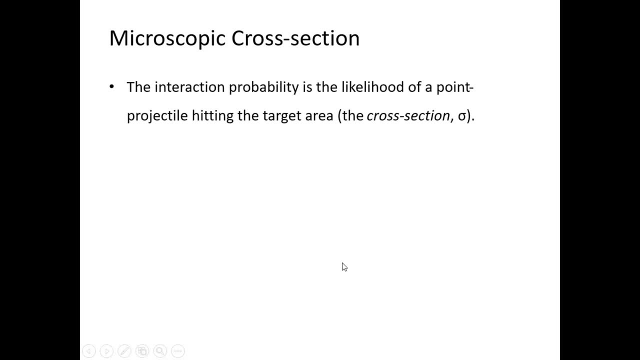 reactions. So to find and estimate how the reactions are really carried, and then what neutrons can do, we have to learn how the, how the number of reactions are taking place. and one interesting quantity is the microscopic cross section. Microscopic cross section for the nuclear. 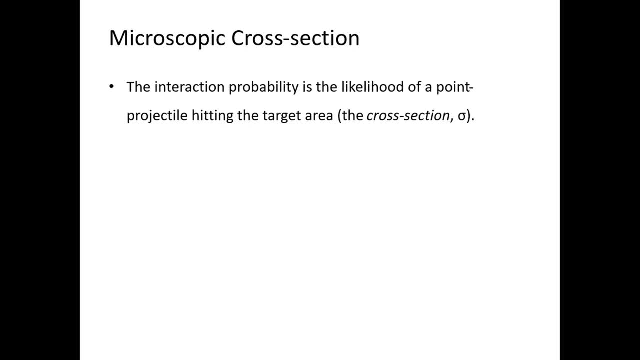 reactions, particularly in the case of neutrons, is really interesting. So so, microscopic cross section is basically interaction probability. It is the likelihood of a point projectile-like hitting the target area, the cross-section, and how much target area a point projectile sees. 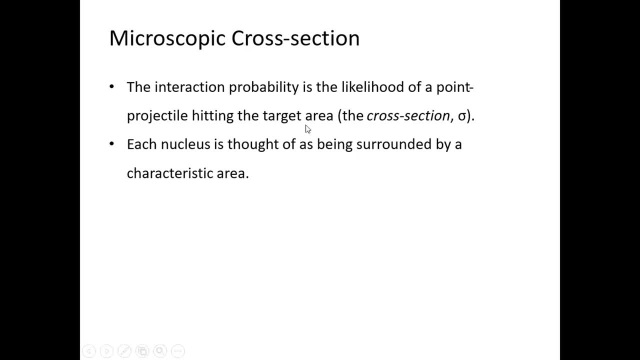 each nucleus is thought of being is surrounded by certain characteristic area which may be larger or smaller than the: the area of the, the physical area of the nucleus. the measurements are done in the terms of areas and the smallest term used is bond, which is 10 to the power minus 28 meters square. 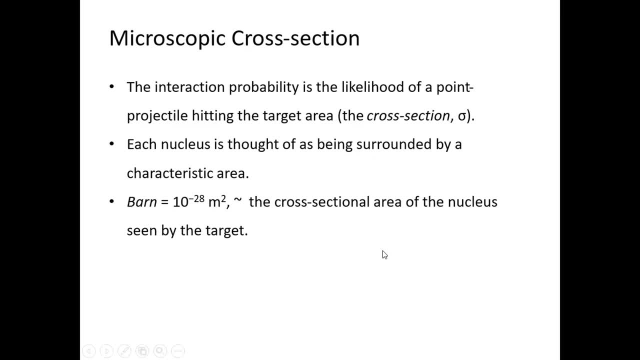 or in terms of centimeters, one bond is equal to 10 to the power, minus 24 centimeters square. it is the cross-sectional area of the nucleus that is seen by the target hitting neutrons. the cross-sections are different, so neutron sees different cross-sections for different processes. 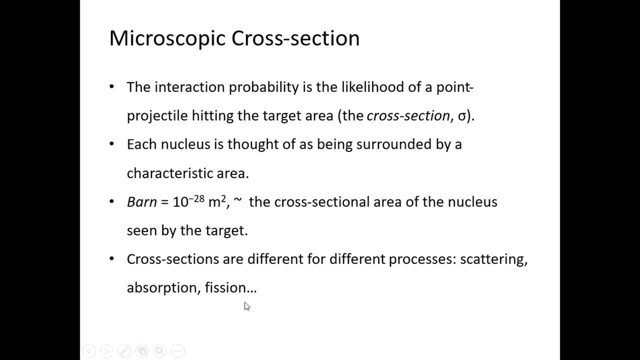 for example, if it is scattering it sees different area. if it is absorbing, it sees different area of the same nucleus, it sees extremely different. proficient. the cross-sections are not constant quantities. they are dependent on energies. the incident: neutron energy. if you change the, the, the slow neutrons of the fast neutrons are hitting, then the cross-section change which. 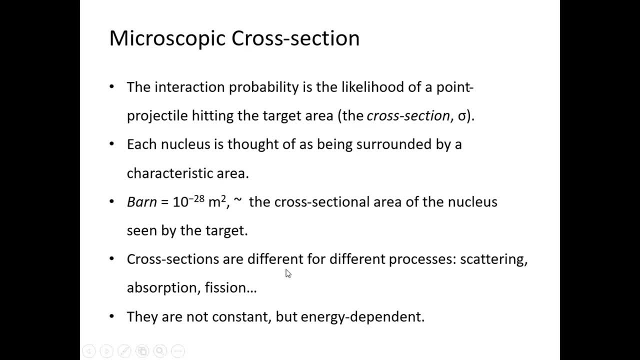 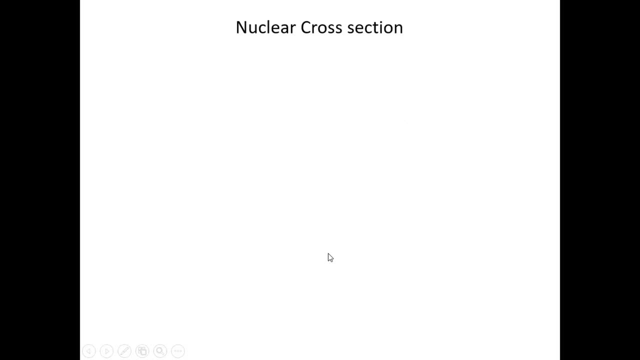 means the possibility of the reaction changes, the probability of the reaction changes, because interaction probability is uh proportional to the cross-section seen by the, the nucleus, the nuclear cross-section. uh, if i, if i briefly to explain this in terms of, of, uh, of a real reaction, then we can guess a beam. 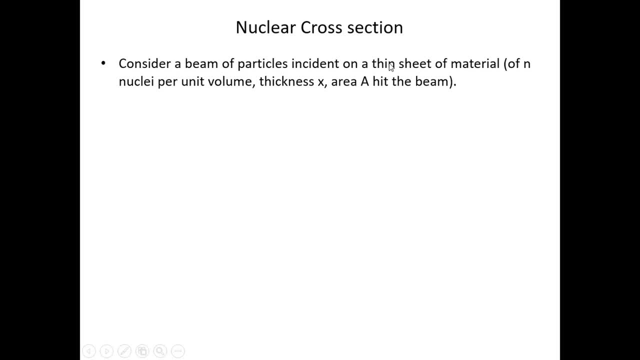 of uh particles that are hit. that is really hitting a thin sheet of material which is containing n number of nuclei per unit volume. that is n per centimeter cube and the thickness is x or d x. the area is a which is hit by the beam. so if one particle interacts only with the dn. 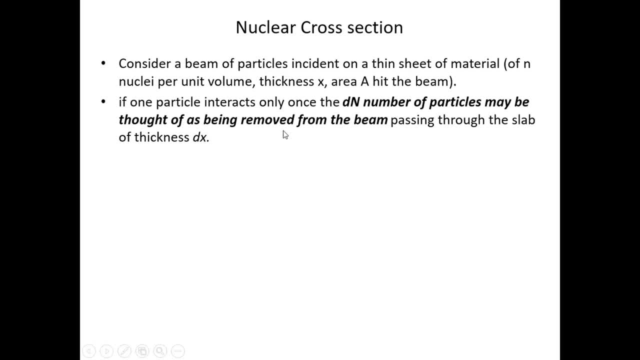 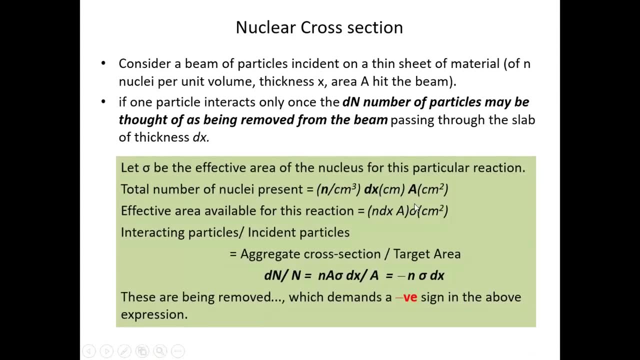 number of particles throughout this as being removed from the beam and passing through the slab of the thickness dx. then we can find out the effect of area Area. the total number of nuclei present can be estimated with the help of this: n is the total number of particles per. 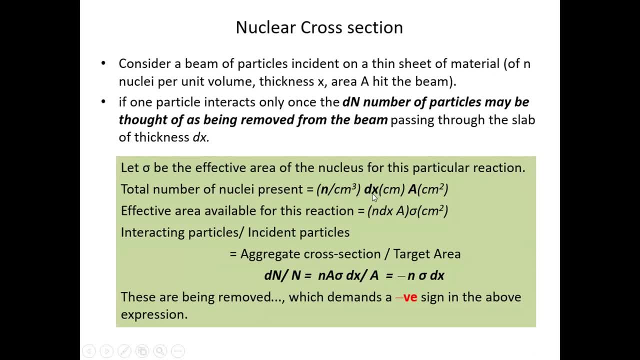 centimeter cube per unit volume. and if you multiply by dx multiplied by a, this is the volume exposed- then we get the number. the total number of the nuclei and effective area which is available for the reaction then is n dx into a this, this total number of nuclei multiplied by each nuclei. 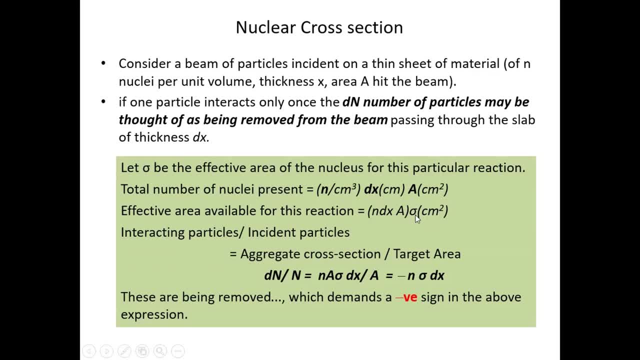 see the sigma, the microscopic cross-section. this is the area seen by each nuclei. so this is the total effective area available for the reaction. so interacting particles per unit. the incident particle is this total divided by the target area and we see that this is given as n multiplied by sigma into dx, and this is what the rate, the interacting 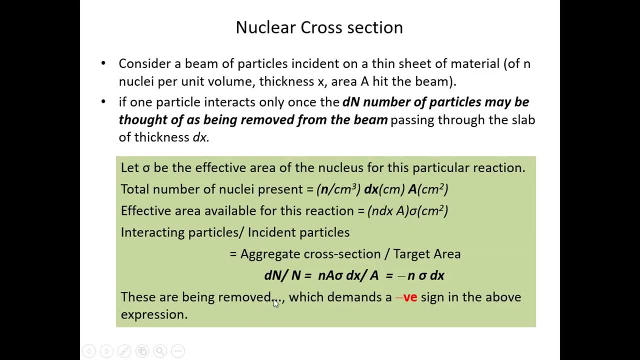 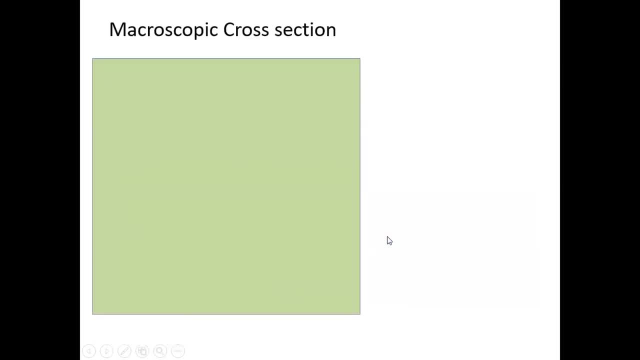 particles per incident particles are and the this is being removed. therefore the negative sign is there. I can further find out the macroscopic cross-sections ideas with the help of this equation, but let me tell you that once we have produced this kind of a product, n into sigma the number 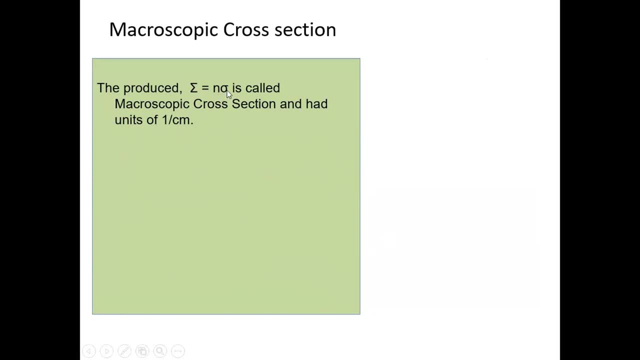 of particles per unit volume multiplied by the cross-section seen by individual neutron, then this is the. this is the macroscopic cross-section, and it is macroscopic cross-section. it has a unit of one over centimeter. it is also called mean free path proportionality, because one over this macroscopic 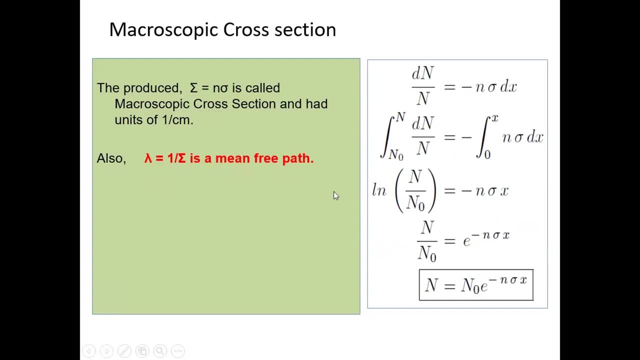 cross-section is the mean free path. as we have already seen, this number of particles that are removed from the bean, per per unit particles, is given by n into sigma, into dx, and this is the macroscopic cross-section and we can integrate it from initial values to to certain value in time. 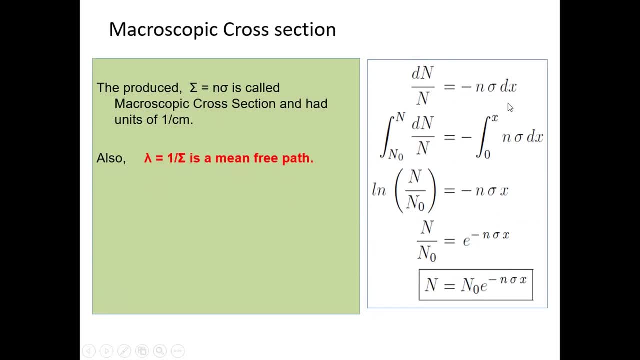 and for zero to x the distance of of a slab. and then if we integrate we get n over n naught times e to the power minus n sigma into x and sigma we can same. it is a macroscopic cross-section so we can write it in the capital sigma: capital sigma multiplied by x. so we can see that it is it. 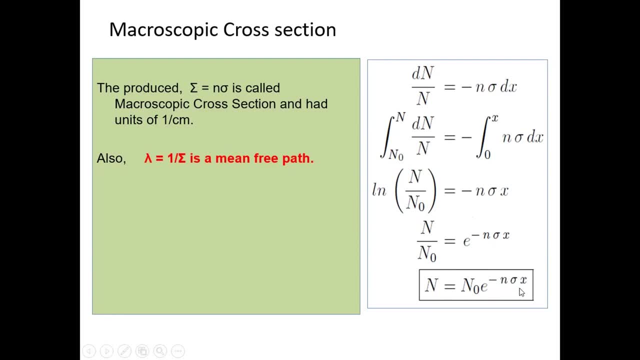 is the number which is removed from the beam is is exponentially changing with the distance. so the the particles that came at the at the beginning of this lab and the particles that are at the end of this lab are really different and they are decreasing by this exponential curve. 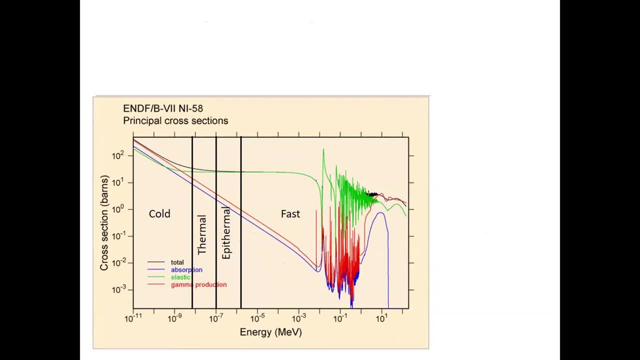 people have shown the measurements through measurements, experimental measurements. the cross sections are really really different for different materials and they are energy dependent cross sections. these are the microscopic cross sections. here i show you that these cross sections are the experimental cross sections. they are fitted with the, with the 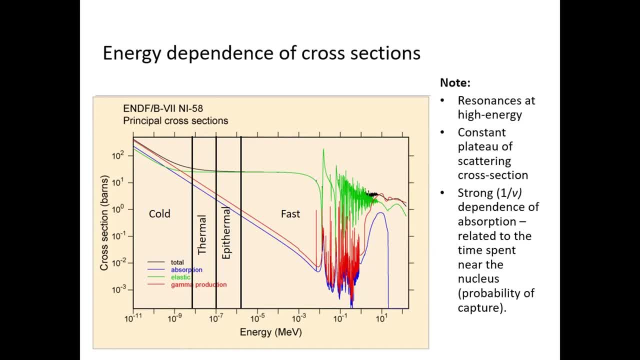 the curves and they show these uh, these uh different uh behaviors. let me i briefly tell you that this is evaluated nuclear data pile which has been produced with the worldwide uh uh help and the all cross-sections are reported there and the experimental cross sections are placed and then a fitted curve is produced. the cross sections are in terms of bonds. 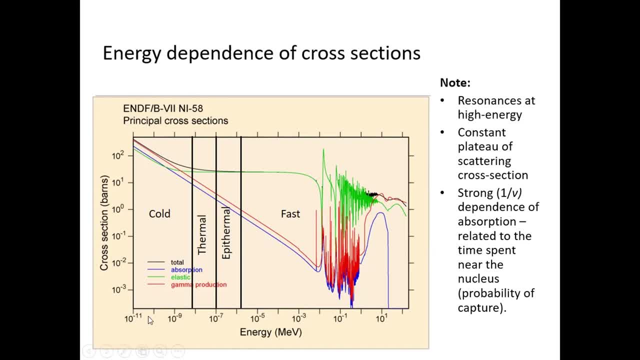 and this is a logarithmic scale on which it is shown on x, x's. the energy is also shown in the logarithmic scale and it is MEV scale. Therefore, 10 to the power minus 6 multiplied by MEV will 10 to the power minus. 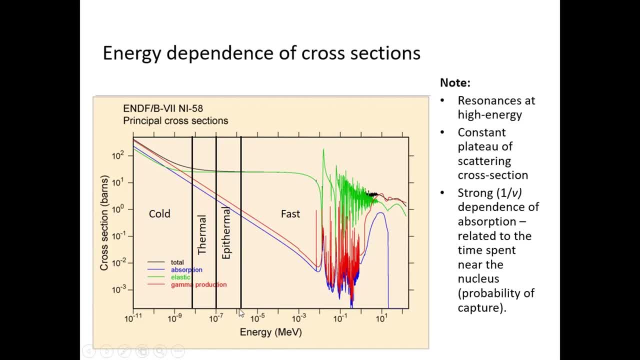 6 multiplied by MEV will make it 1 electron volt. So, roughly speaking, here is the 1 electron volt and the less than 1 electron volts are here and the more than 1 electron volt are there. This is 10 million electron volts. The regions are called the cold region for 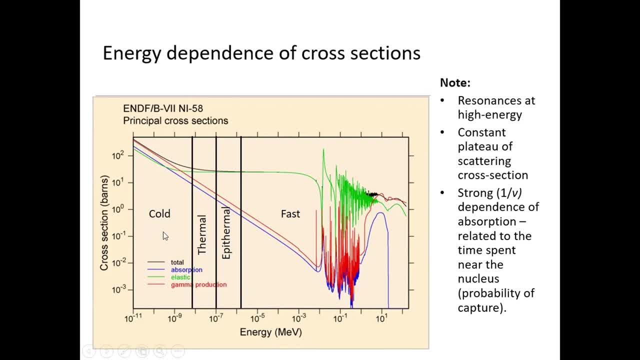 the neutrons. The neutrons in these energy ranges are called cold electrons. The neutrons in the energy range of 0.1 electron volt and less are called thermal electrons, and the epithermal electrons are those lying with the 0.1 to 1 electron volt energy range. and 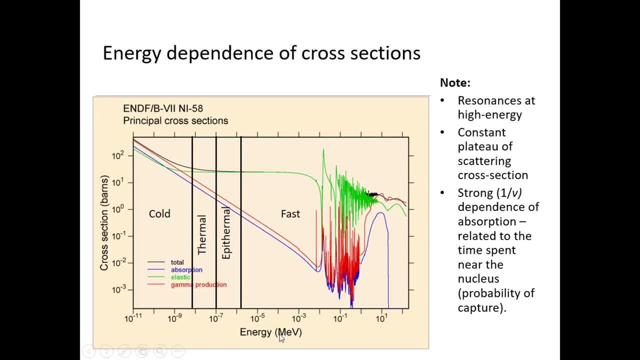 the fast electrons are which have energy higher than 1 electron. It is in tens and hundreds and thousands of electrons. So 10 to the power minus 6 multiplied by MEV is 1 electron volts and less than the million 10 to the power, 7 electron volts, is the possible measured in this graph. the 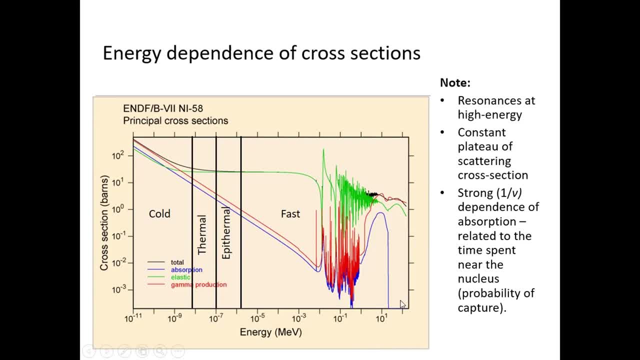 highest possible neutron energy. As you can see, these cross sections are different for the different types of reactions and I will later discuss them, But the regions are according to the energy and their broader names are grouped as cold, thermal, epithermal and fast. 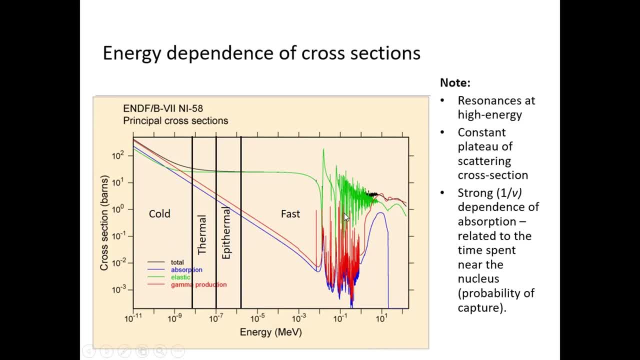 neutrons. The resonances are these: are these sharp changes are the resonances and they occur at the high energy and the constant plateau at the scattering cross section. the fixed values are also shown and 1 over V behavior. is this called the absorption related behavior? 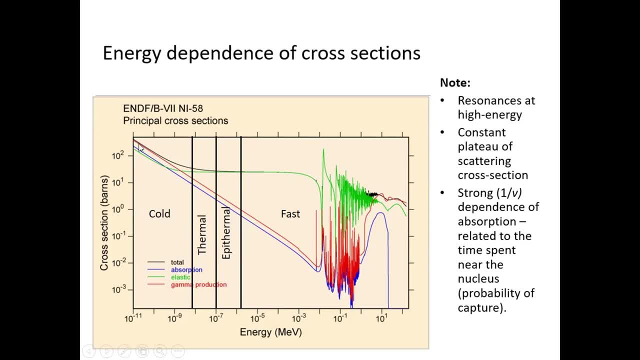 near the nucleus and the probabilities are as 1 over V. V behavior- they call it the straight line decreasing in this kind of a graph. So there are three names for these curves: the resonance region, the constant or the epithermal region. 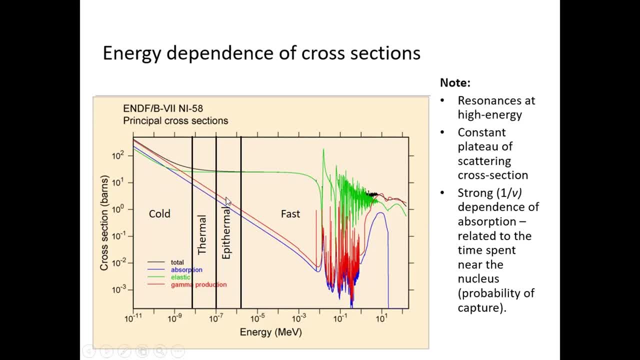 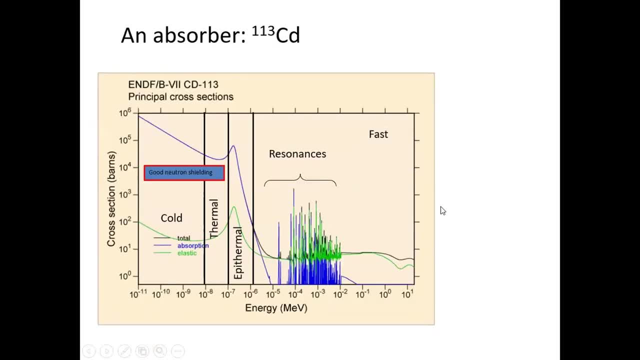 and the 1 over V behavior of the 1 over V dependence of the cross section. Let me I will also very briefly talk about this cadmium. It is generally used as a shielding material and in a current nuclear system they are the absorbers for the neutrons, because they 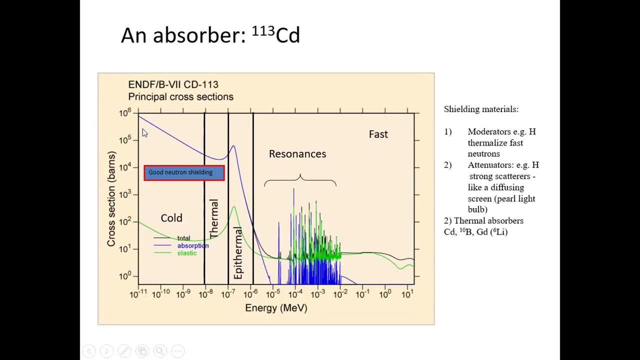 have shown very high cross section for the absorption. This blue curve is the absorption and the thermal- The cold and the thermal region shows this. before this one resonance value. this is the behavior and the resonances are very, very small as compared to this strong absorber. 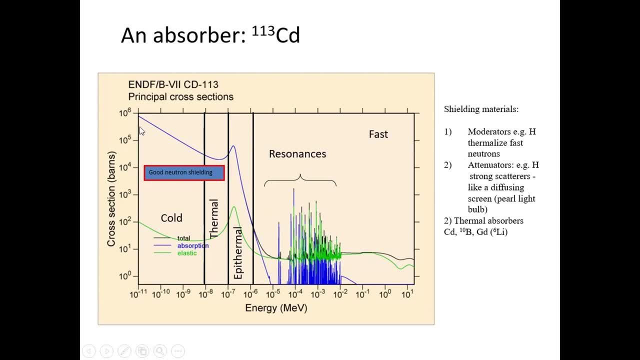 You can see the cross section is about 10 to the power 6 bonds very high cross section in the in the cold and the thermal region and in the epithermal region and the fast region. it it has a resonances So this is a good 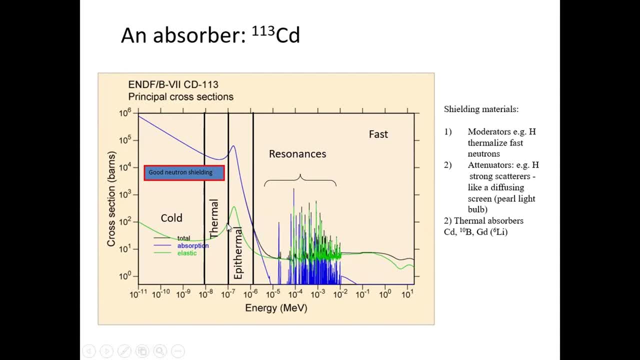 shielding material. if the neutrons are in the thermal region, or or they are epithermal neutrons, or if they are cold neutrons, then this kind of material is the best material. So cadmium, boron, godanium, the lithium 6 are really termed as great absorbers, or 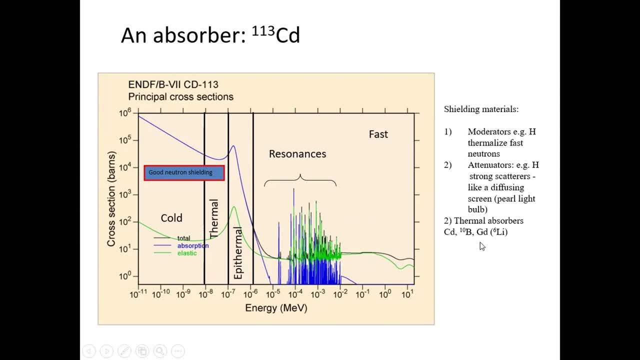 the control materials for the nuclear reactor systems. They scatter strongly, They diffuse strongly, They also absorb strongly. And here we show the elastic scattering curve and the, the absorption, the curve, and they, they are really very good absorbers, and that's how the neutrons